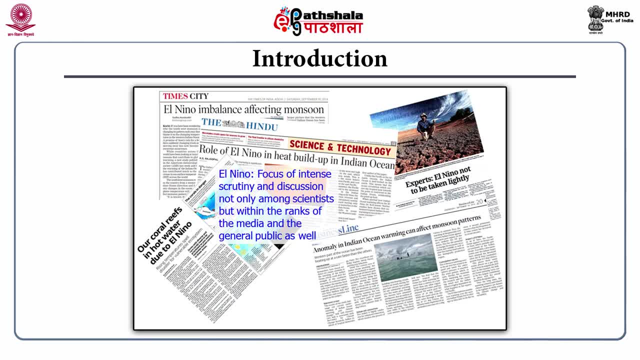 Long-term East Pacific sea ubiquity is an invitation to see the entire bear Today mid-イآ. nature will be adjustment and other conditions around which the Bastuan Sea will remain Past. events of these features are easy. high floor conditions where the water should. 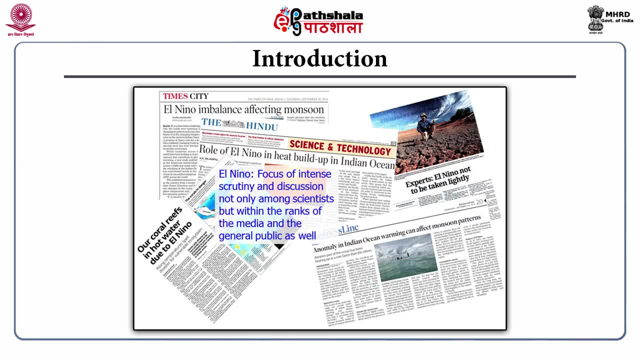 have level surface impact caused by rains and, at some point of the season, the Mesra and the Meru tuhin bore should have exactly the same results as the Hanmeh, specifically with the global meteorological situations which are technically called as Southern Oscillations. 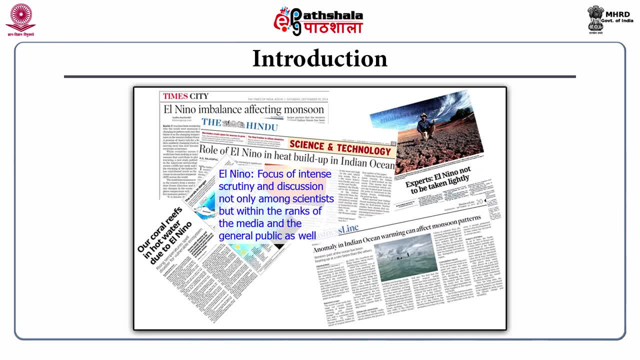 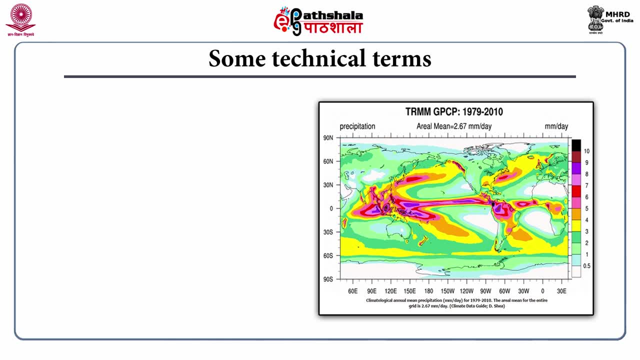 Together, El Nino and Southern Oscillation are known popularly as NSO. Now let me explain some of the technical terms that I shall be frequently using during this discussion. it is a quantitative description of values of a climatic variable averaged over a period of time. 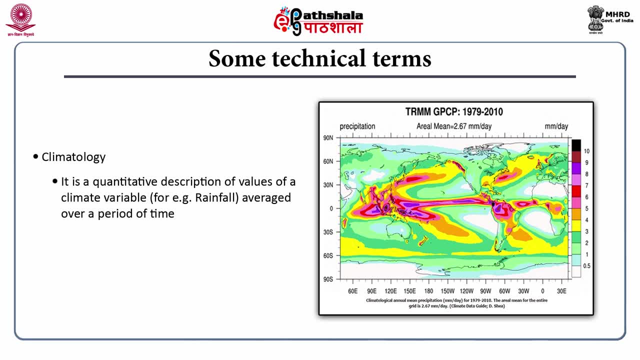 For example, a case of rainfall has been given here. From this figure we can say that the rainfall over most locations of the oceans are, in general, higher than the land masses. it is a mass motion in a field, resulting in transport and mixing of the field. 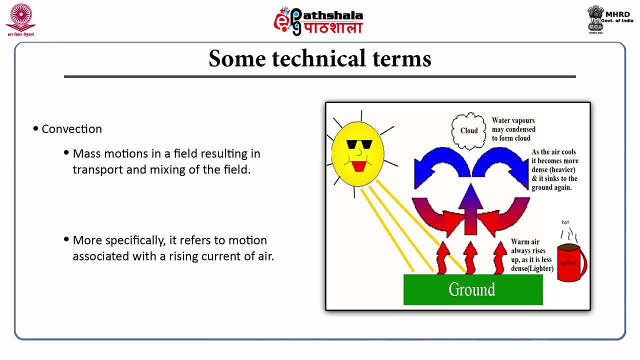 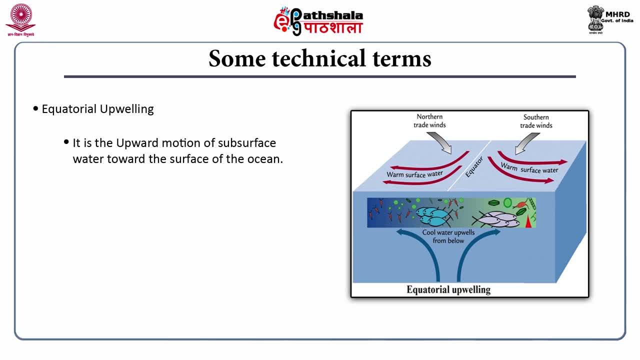 More specifically, it refers to motion associated with a rising current of air, Then equatorial upwelling. It is the upward motion of subsurface water toward the surface of the ocean. This is often a source of cold and nutrient-rich water. Strong upwelling occurs. 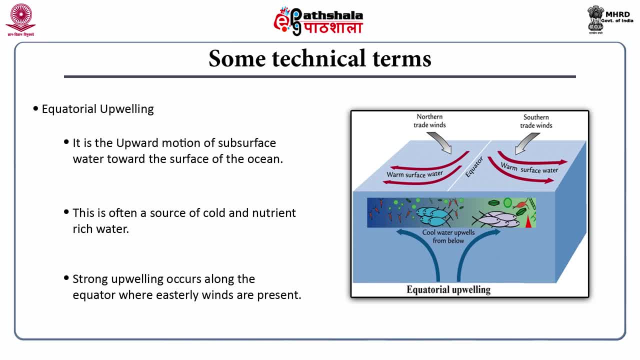 It can be expressed with a gravitational force of of a spring-, ikke wind. All should be represented and defined as topical. because temperature changes. This is a function called thermocline. This is a thin but distinct layer in a large body of fluid like ocean or lake. 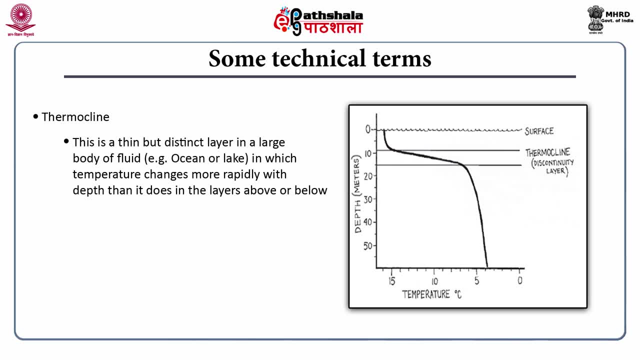 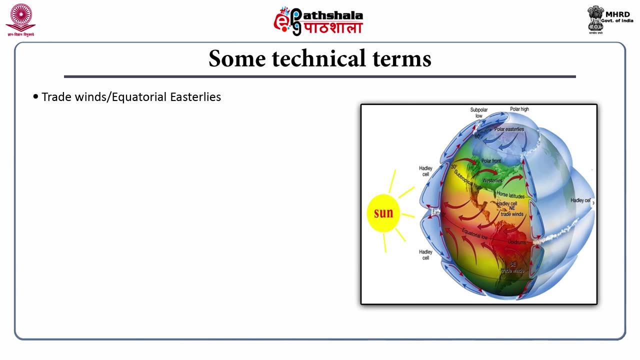 So in this layer temperature changes more rapidly with depth than it does in the layers above or below. It forms when water at the surface of an ocean or lake is heated up while the water below that layer stays cool. Now trade winds or equatorial stirrleys. 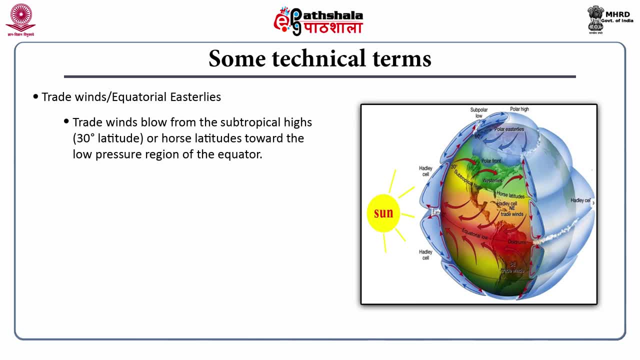 Trade winds blow from the subtropical highs about 30 degree latitude, or also called horse latitudes. So these winds blow from this subtropical highs towards the low pressure region of the equator. They are named from their ability to quickly propel trading ships across the ocean. 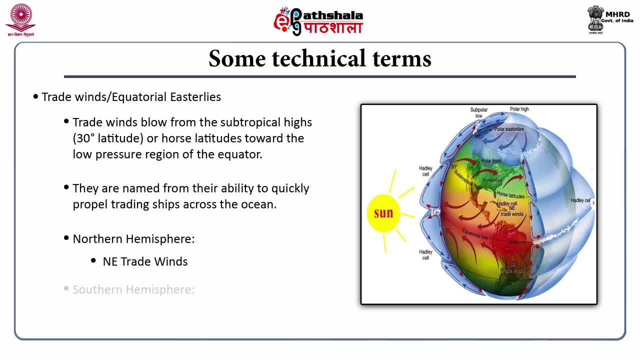 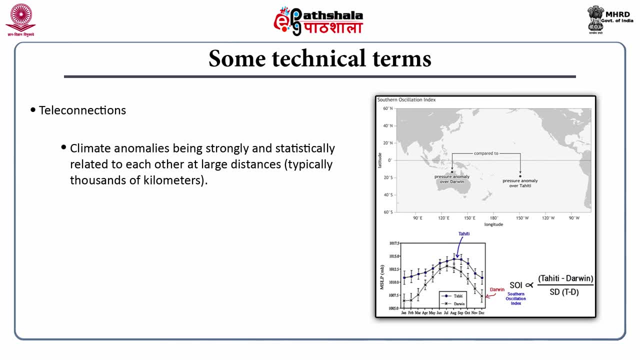 In northern hemisphere trade winds are northeasterly and in southern hemisphere trade winds are southeasterly. Teleconnections, climate anomalies being strongly and statistically related to each other at large distances, typically thousands of kilometers. Take, for example, linkage of sea level pressure at Tahiti in the Pacific Ocean and Darwin. 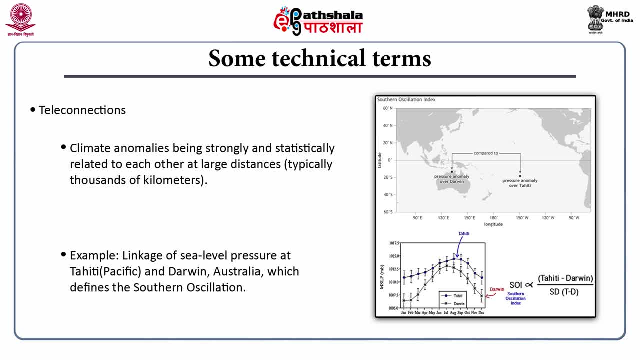 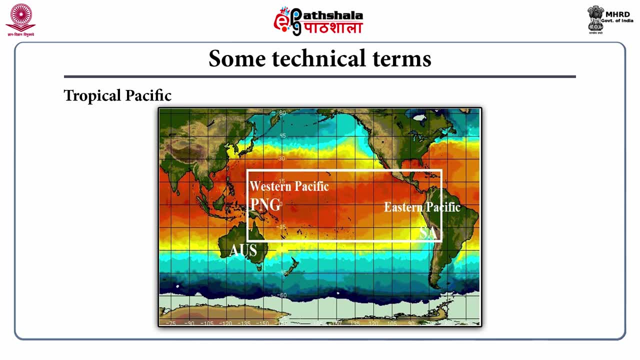 port of Australia. This defines the southern oscillation, Now tropical Pacific. when you mention of tropical Pacific in the NSO context, we are talking about the region marked by red in this figure. In the western part of the tropical Pacific, we are talking about the region marked by red in this figure. 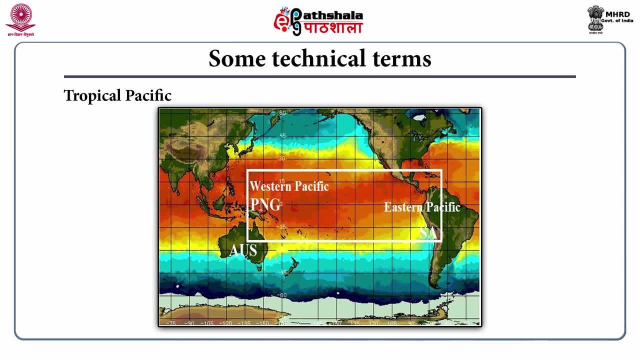 In the western part of the tropical Pacific. we are talking about the region marked by red in this figure. In the southern part of the tropical Pacific, there is countries like Indonesia, Philippines and Australia, whereas in the eastern part, there are countries of Central and South America. 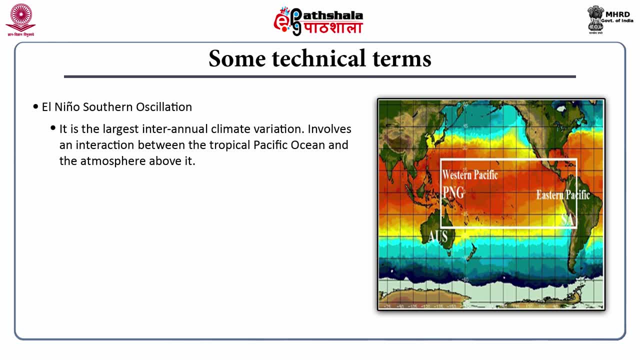 El Nino and the Southern Oscillation. It is the largest interannual climatic variation. It involves an interaction between the tropical Pacific Ocean and the atmosphere above it. Its impacts are felt worldwide. Heart of the NSO lies in the tropical Pacific Ocean along the equator. 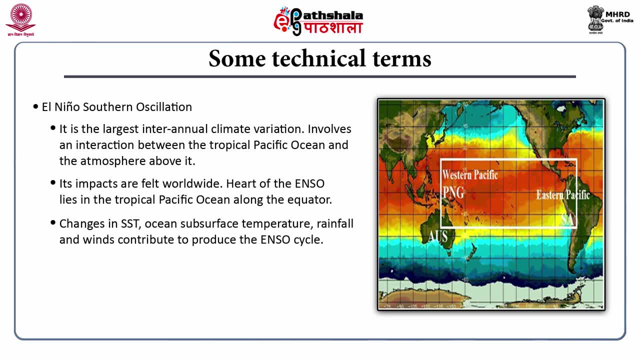 Changes in SST, that is, Sea Surface Temperature, temperature, ocean subsurface temperature, rainfall and winds contribute to produce the NSO cycle. The variations in the Pacific basin within about 10 to 15 degree latitude of the equator are the primary variables driving this NSO process. 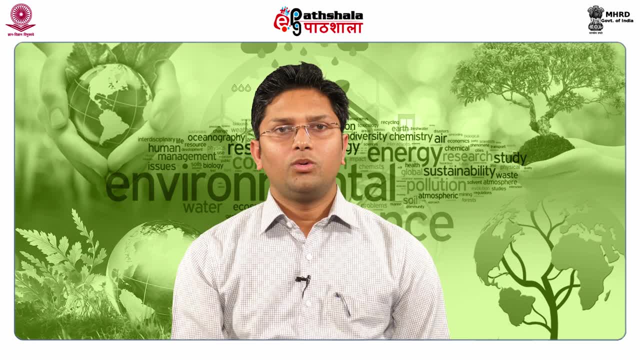 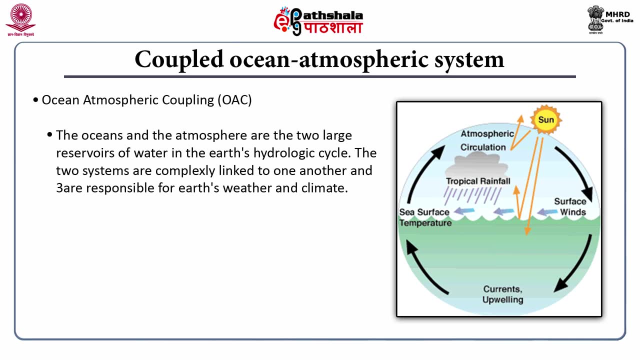 In the few subsequent slides we shall discuss the coupled ocean atmospheric system. Ocean atmospheric coupling. the oceans and atmosphere are the two large reservoirs of water in the earth's hydrological cycle. The two systems are complexly linked to one another and are responsible for earth's weather. 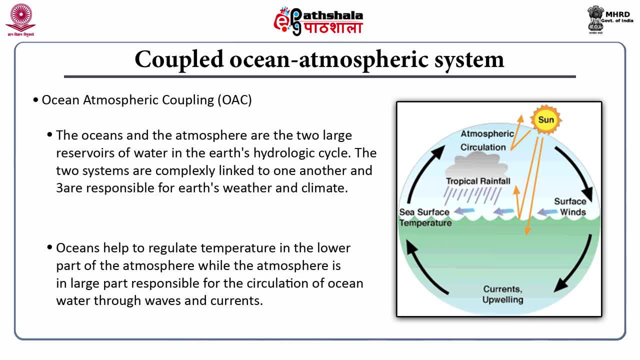 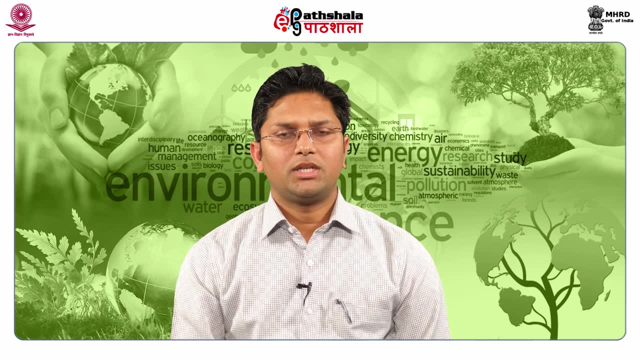 and climate. Oceans helps to regulate temperature in the lower part of the atmosphere, while the atmosphere in large part responsible for the circulation of ocean waters through waves and currents. Now let me tell you the theory behind the ocean atmospheric coupling. A large scale anomaly of sea surface temperature induces diabetic heating or a global warming. 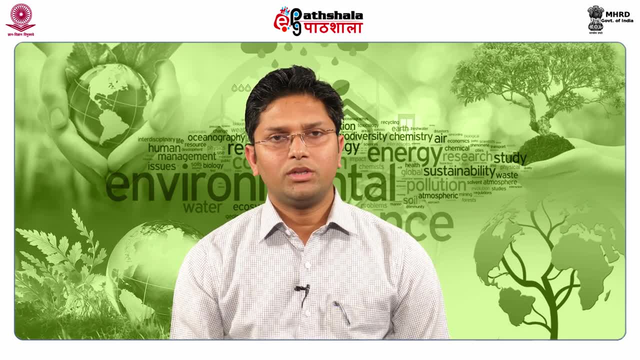 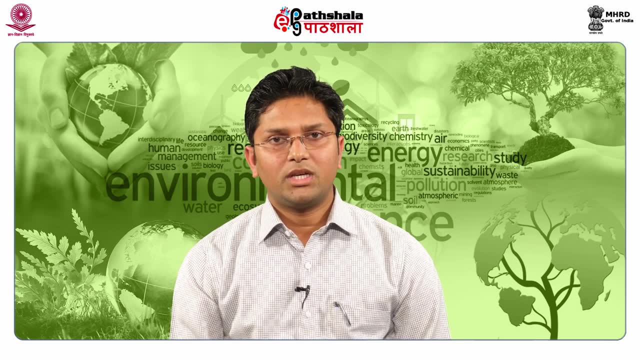 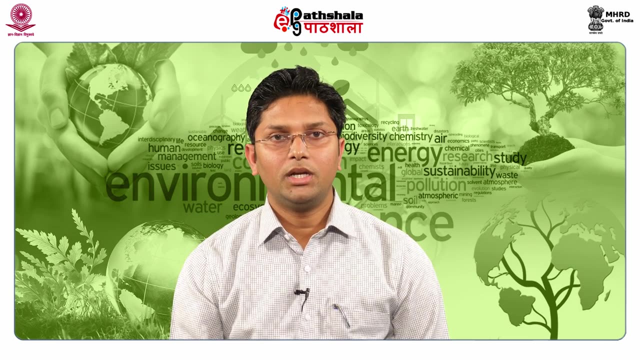 or cooling of the atmosphere, which changes atmospheric circulation and hence the wind distress and heat fluxes at the ocean surface. As a result, ocean thermal structure and circulation gets modified, giving rise to a series of positive feedbacks that strengthen the initial SST anomaly. 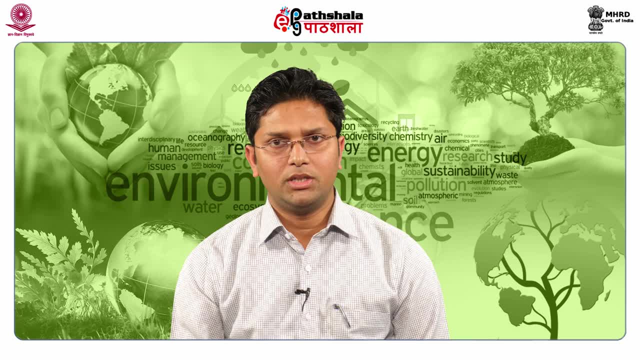 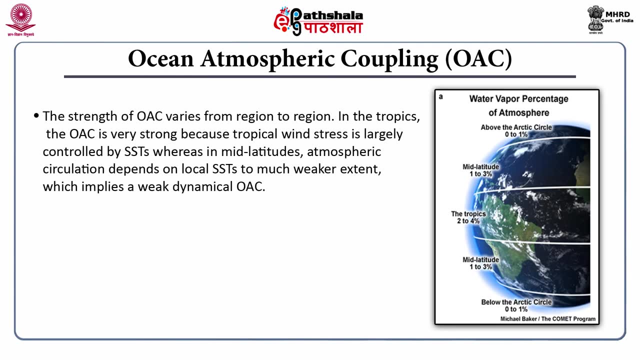 Ocean and atmospheric circulations are interdependent on each other and the SST serves as a link combining these two elements. The strength of ocean atmospheric coupling varies from region to region. In the tropics, the coupling is very strong because tropical wind stress is largely controlled. 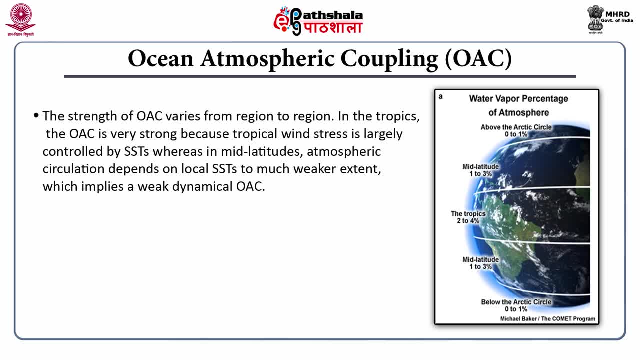 by sea surface temperature, whereas in middle latitudes atmospheric circulation depends on local SSTs and the dependence is weaker. So El Nino is a warm phase of a natural oscillation driven by tropical ocean atmospheric coupling, and perhaps this is the case. This is the most striking example of active coupling. 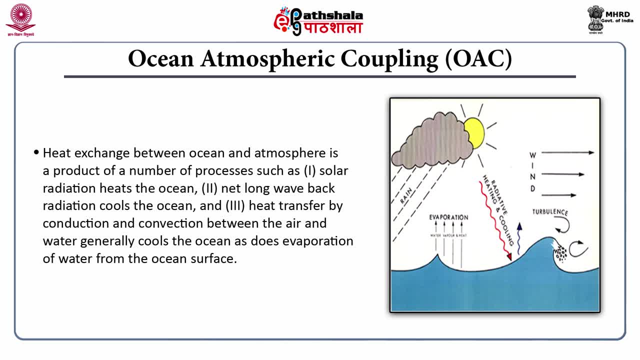 Heat exchange between ocean and atmosphere is a product of a number of processes such as: solar radiation heats the ocean, then ocean radiates back long wave radiation. This process cools the ocean. Then heat is transferred from the ocean to the atmosphere by way of conduction and convection. 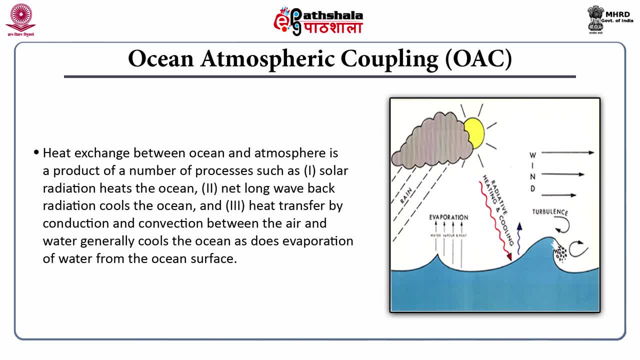 Also, there is evaporation from the ocean surface, and this evaporation process cools the ocean. In the few subsequent slides we shall elaborately discuss the following processes. First, the evaporation process. The evaporation process is the process of cooling the ocean. 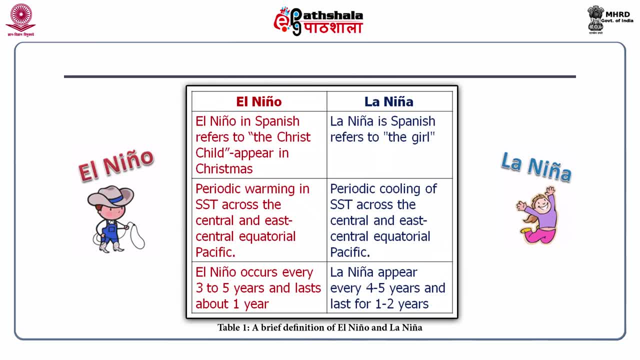 Then the cooling process, Then the cooling process of the ocean, Then the cooling process of the ocean. This is the end of the first slide. but the cooling process is similar to the cooling process of the ocean. The cooling process of the ocean happens for the recent years as well. 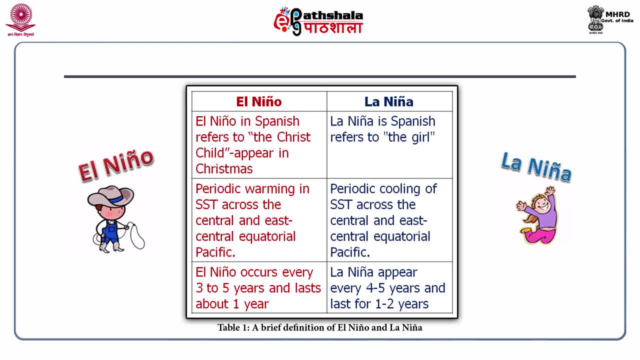 We are going to discuss about El Nino and La Nina. This table gives a brief definition of El Nino and La Nina. El Nino and La Nina are Spanish words. El Nino means the Christ child which appears in Christmas, And La Nina is the girl child. 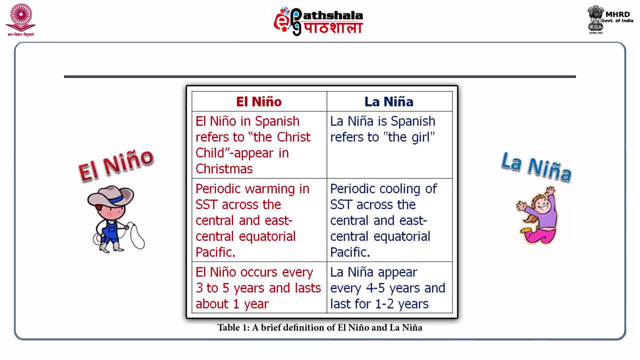 In case of El Nino, there is periodic warming in the sea surface temperature across the Central and East-Central equatorial Pacific. In case of La Nina, instead of warming, there is periodic cooling. in the same region, El Nino occurs every 3 to 4, 5 years. 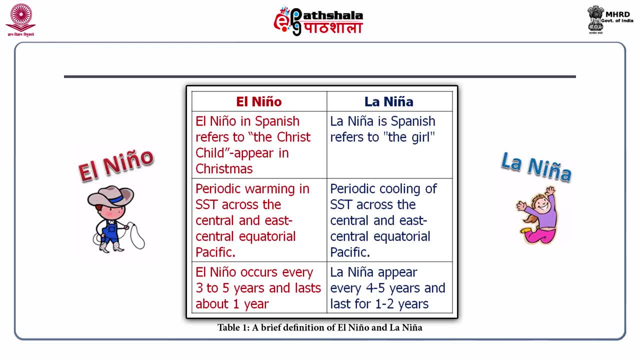 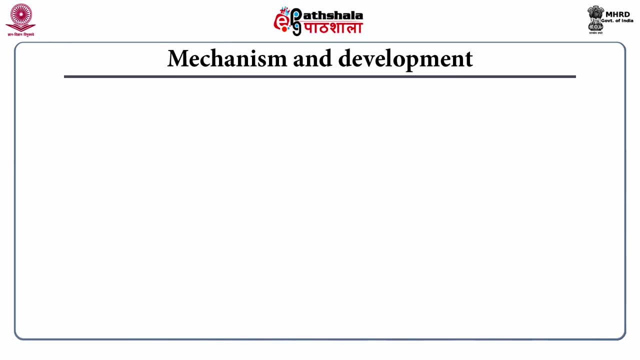 years and last about one year, whereas La Nina appear every four to five years and last for one to two years. Now the mechanism and development of El Nino and La Nina. First, let us see how pressure plays a role in it In case of normal air. 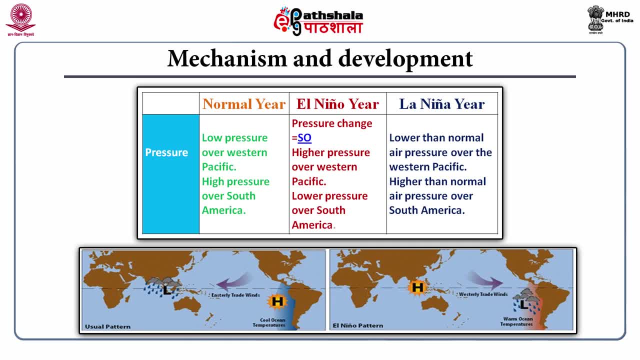 there is low pressure over western pacific region and high pressure over eastern pacific region, that is, south American region. In case of La Nina, this pressure changes and this is called southern oscillation. That is, during El Nino air you will find higher pressure. 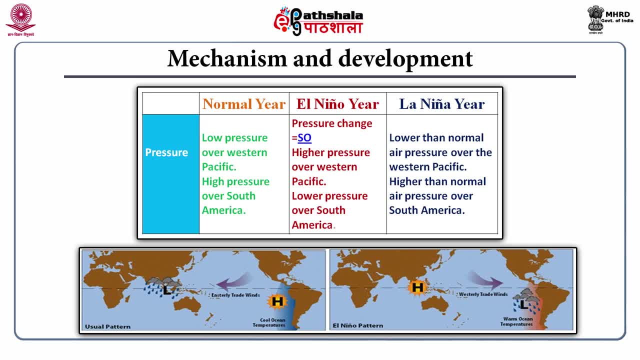 over western pacific region and lower pressure over south American region. In case of La Nina air, it will be normal air but the magnitude will be higher, that is, the air pressure over the western pacific will be lower than its normal and the pressure over the south America. 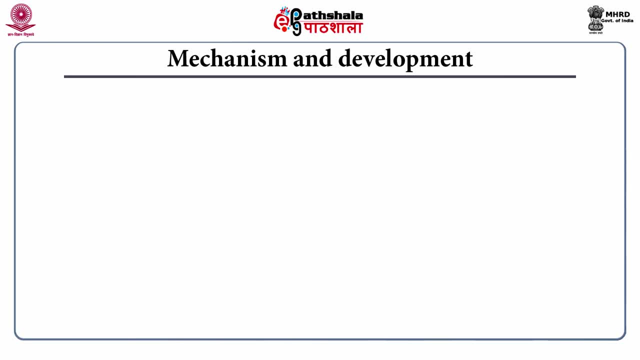 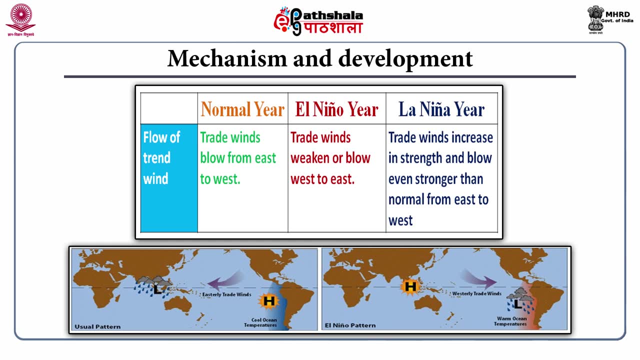 will be higher than the normal value. Then flow of trade. In normal air trade winds blow from east to west in the equatorial pacific region, that is. the wind blows from south American side to the Indian Ocean sides and along the wind the ocean water also moves towards the western pacific region. That is why in a normal air, 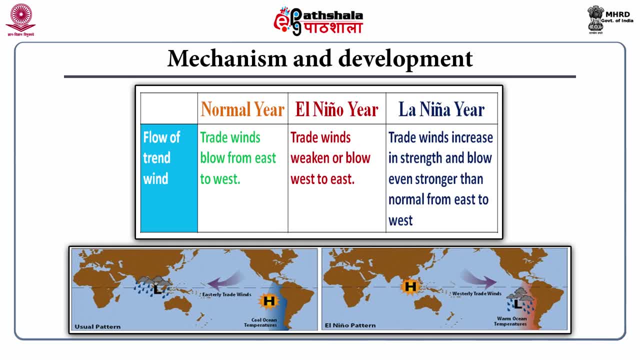 you will find a higher sea level in the western pacific region than that of eastern pacific region. During El Nino air trade, winds either weaken or blow from west to east. In case of La Nina air, the winds are sterling only, but the magnitude or strength is higher. 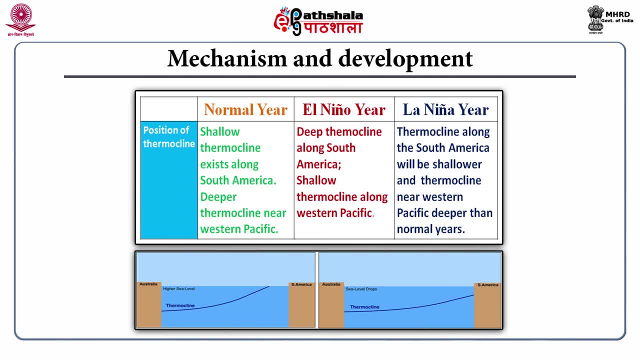 Now the position of thermocline In a normal air. there exists a shallow thermocline along south American coast and deeper thermocline near the western pacific region. In El Nino air the thermocline in the south American side gets deeper and the western pacific side gets slower. In case of La Nina air, the thermocline along the south American пл. Erna and traühr van bergen, El Nino Mauss, is under danger. Ahí do появl Mitarbaby plringes. harMAN Perovured to. 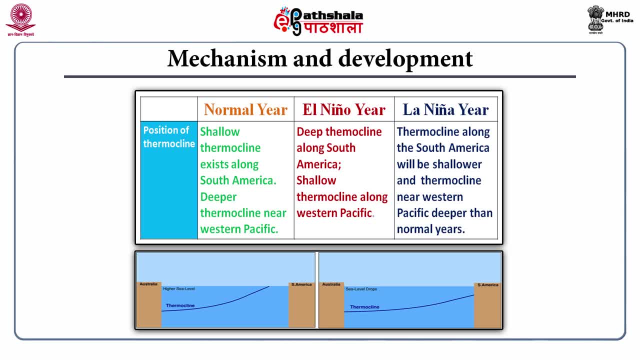 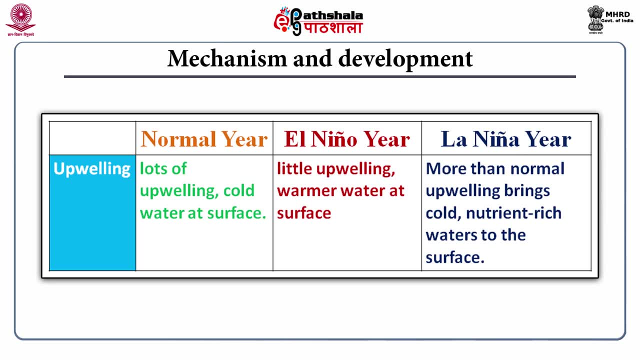 along the South America will be shallower and thermocline near Western Pacific is deeper than the normal years Now upwelling. In a normal year there is a lots of upwelling that is moving of cold water from the underneath of the ocean to the surface. 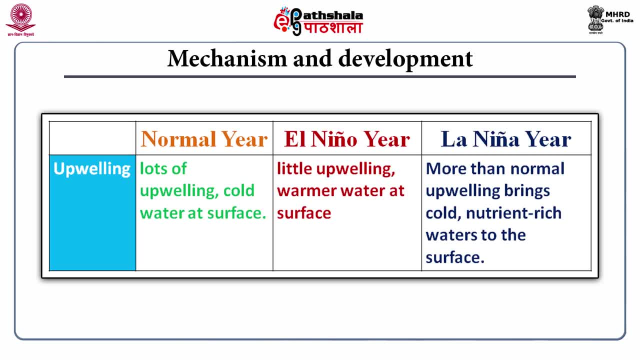 And this upwelling happens off the coast of South America, that is, the Eastern Pacific region. In case of Illinois year, there will be either little upwelling or no upwelling, And the water at the ocean surface will be warmer. For a La Nina year, the upwelling of the Peru coast or the Eastern Pacific region will be 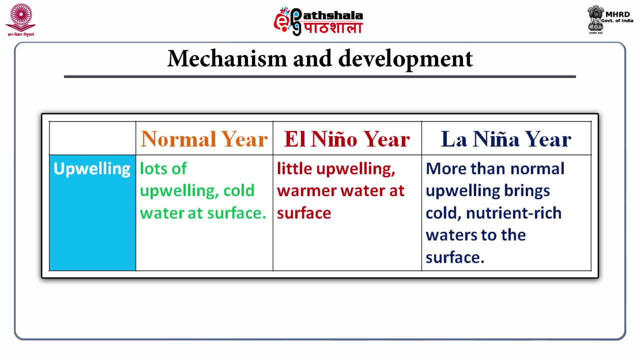 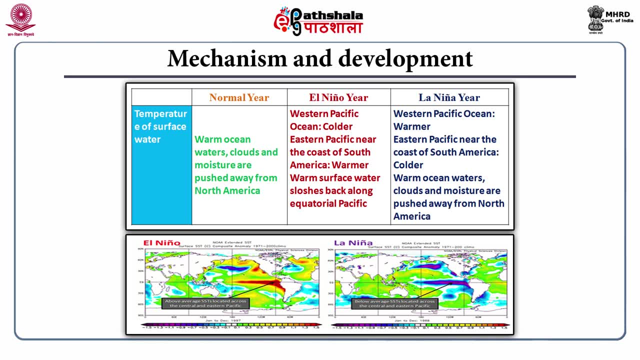 more than the normal, And this upwelling brings cold, nutrient-rich water to the surface. Now let us see what role temperature plays in this El Nino-La Nina development. In normal year, warm ocean water, clouds and moisture are pushed away from North American. 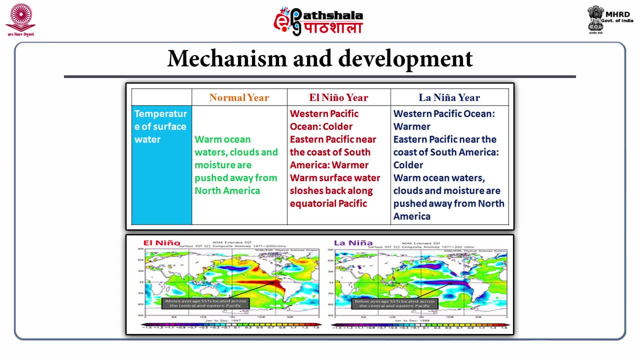 side. In El Nino year, Western Pacific Ocean is colder and Eastern Pacific near the coast of South America Warm. surface water slows back along the equatorial Pacific In a La Nina year. Western Pacific Ocean remains warmer, whereas the Eastern Pacific near the. 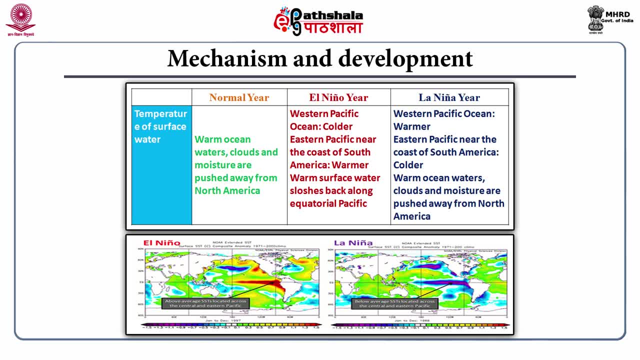 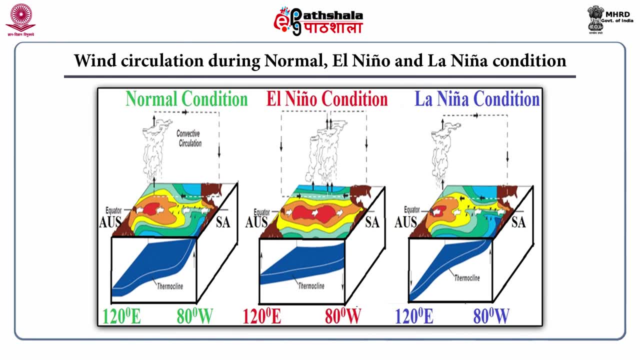 coast of South America is colder. Warm ocean waters, clouds and moisture are pushed away from the North American side. This figure shows the wind circulation pattern both at the surface level and at higher altitude during normal El Nino and La Nina years, And this is in the atmosphere over tropical Pacific. 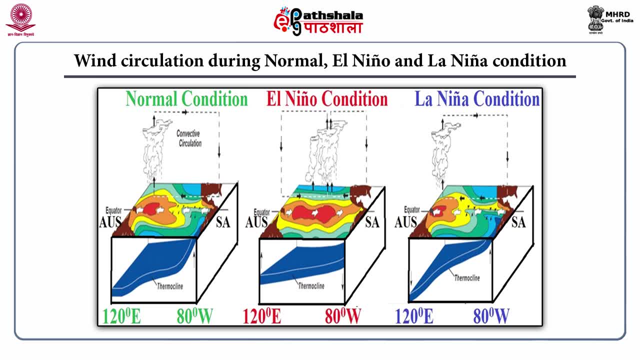 And the region bounded by 120 degree east longitude and 80 degree west longitude. The associated changes in ocean current, then shape of the thermocline and zones of strong convective precipitations are also depicted here, Like in a normal condition. in a normal year the convective precipitations are generally 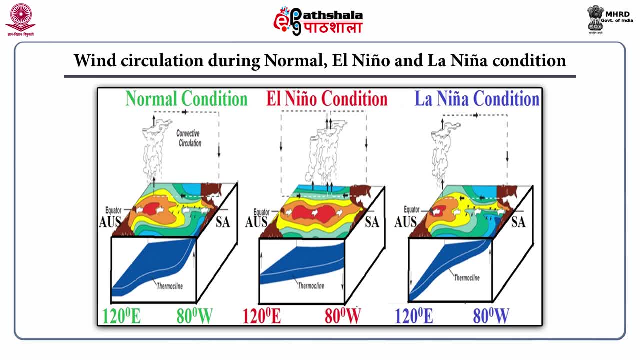 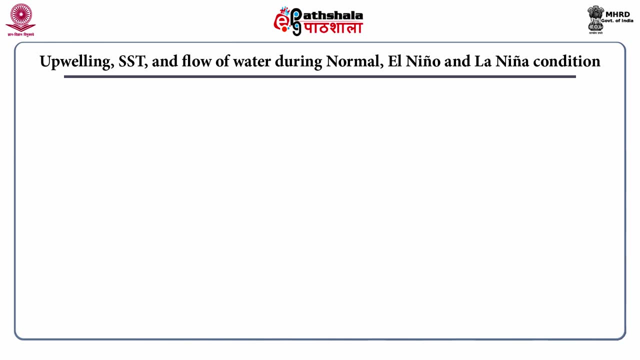 in the Western Pacific region. In the La Nina years that ships far of the Western Pacific And in case of El Nino year, either it is in the Central Pacific region or towards the Pacific eastern pacific region. upwelling sea surface temperature and flow of water during normal. el nino and la nina condition. these figures have been taken from the reports of tropical ocean atmospheric project. during a normal year, the surface height is more. in the western pacific sea, surface temperature is higher and there is upwelling of cold water near the south american. 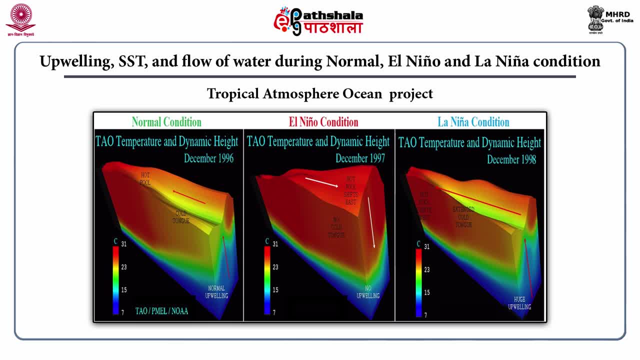 coast, that is, in the eastern pacific region. during el nino year overall, tropical pacific is warmer, sea level and temperature is higher in the eastern pacific region and there is no upwelling during la nina year. overall, the ocean is cooler than normal. western pacific is warmer and there 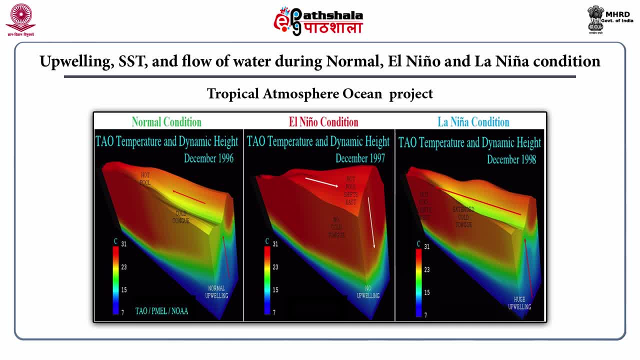 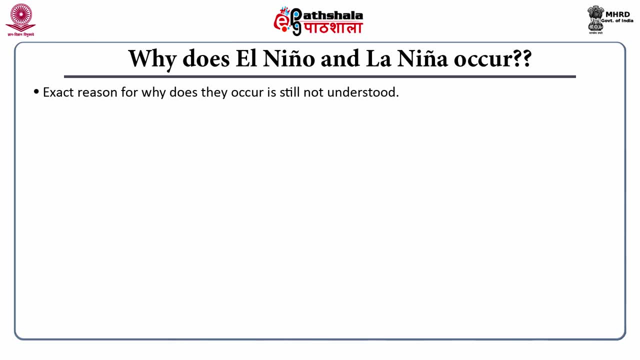 is a huge upwelling of the of the peru coast. that is huge upwelling in the eastern pacific region. let us look at the reason why does ellinoc assimil peanuts occur? exact reason for why does they occur is still not understood. ellena results from interaction between the surface layers of the 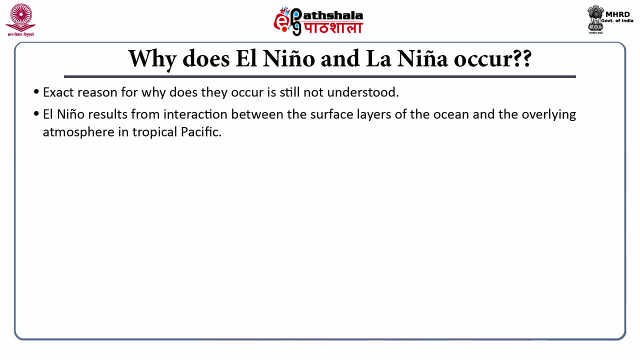 ocean and the surface layer of ocean idol, and from there it matches the dynamic of the ocean between the overlying atmosphere in the tropical Pacific region. It is the internal dynamics of the coupled ocean atmosphere system that determine the onset and termination of El Nino. 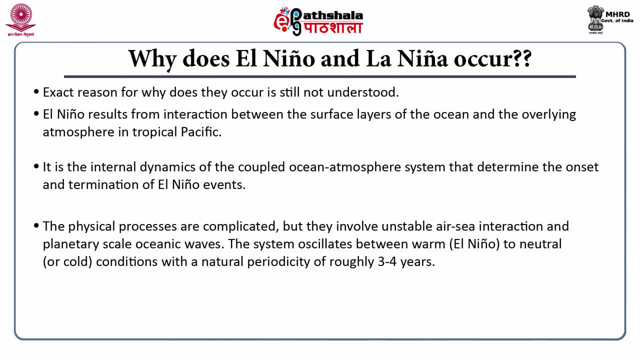 The physical processes are complicated, but they involve unstable air-sea interaction and planetary scale oceanic wave. The system oscillates between warm, warm phase, that is El Nino phase, to neutral or cold phase, that is, La Nina phase, with a natural periodicity of roughly about 3 to 4 years. 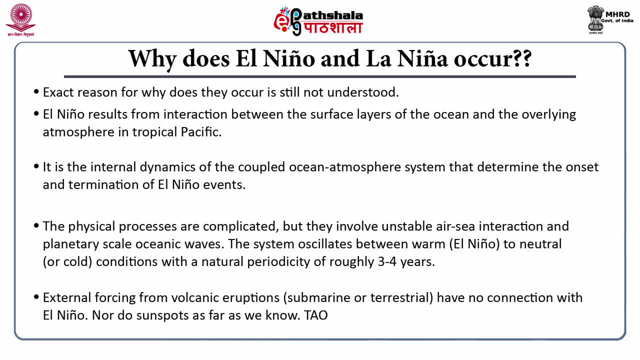 External forcing from volcanic eruptions have no connections with El Nino. Also, sunspots: as far as we know, there is no role of sunspots in bringing El Nino or La Nina. In the next slide we shall discuss how NSO, that is, El Nino and southern oscillation events. 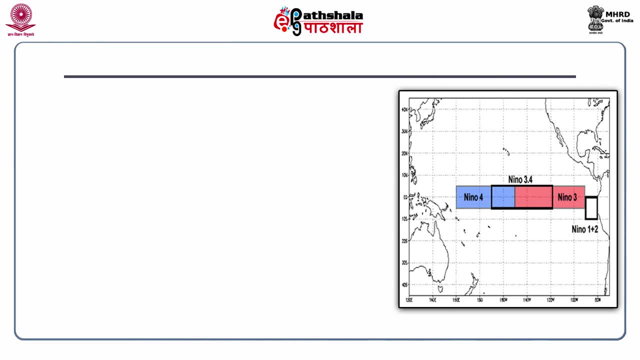 are monitored. This El Nino and La Nina events are monitored with the help of some indices. These are like Nino 1 plus 2, Nino 3, Nino 3.4, and Nino 4.. Like in case of Nino 1 plus 2,, this region typically warms first when an El Nino event. 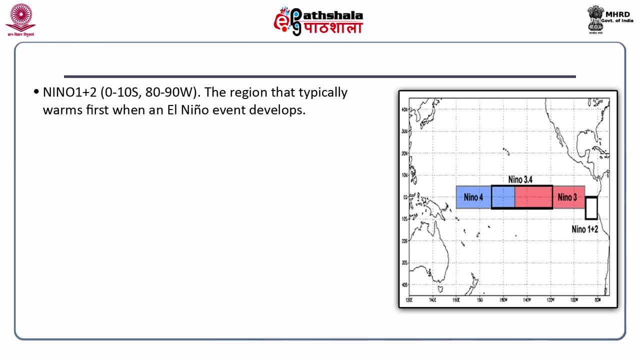 develops, And the observations are taken between 0 to 10 degree south latitude and between 80 to 90 degree west longitude. region Nino 3, the region of the tropical Pacific that has the highest variability in sea surface temperature on El Nino time scales. the observations are taken between 5 degree south latitude. 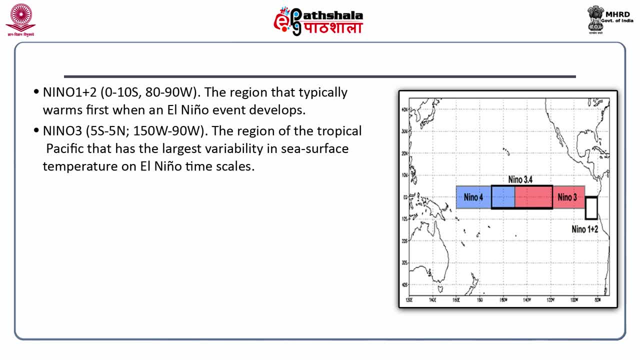 to 5 degree north latitude and between 150 degree west to 90 degree west longitude. Nino 3.4,. for this index, the region defined is 5 degree south to 5 degree north latitude and 170 degree west to 120 degree west longitude. 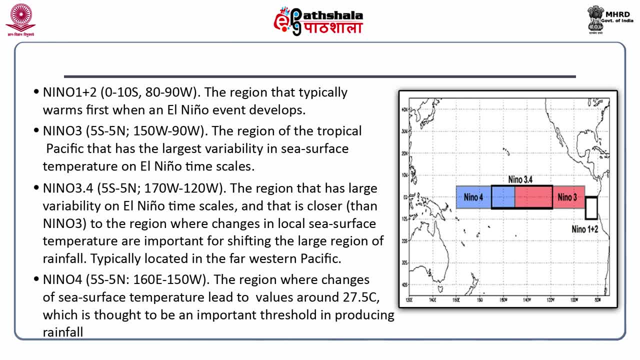 This region is typically located in the far off western Pacific, Then Nino 4,. here the region defined is 5 degree south to 5 degree north latitude and, as per longitude, 160 degree to 150 degree west longitude longitude. This is the region where changes of sea surface temperature lead to values. 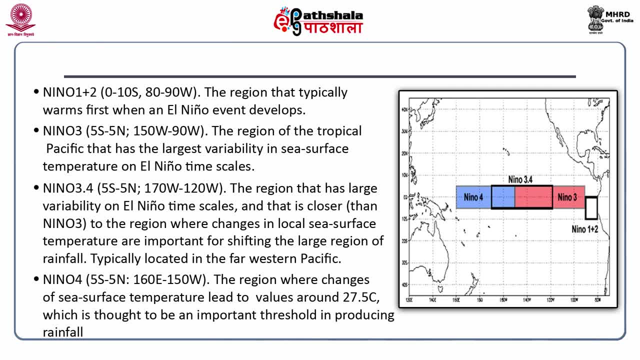 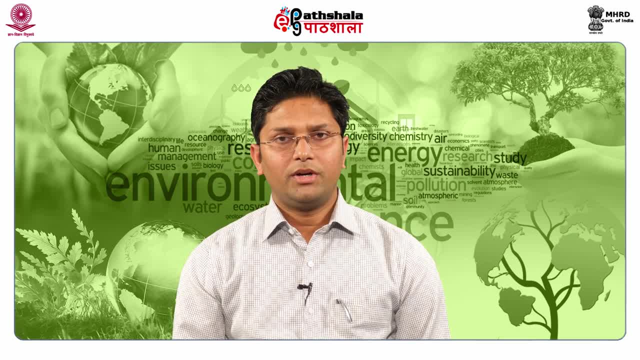 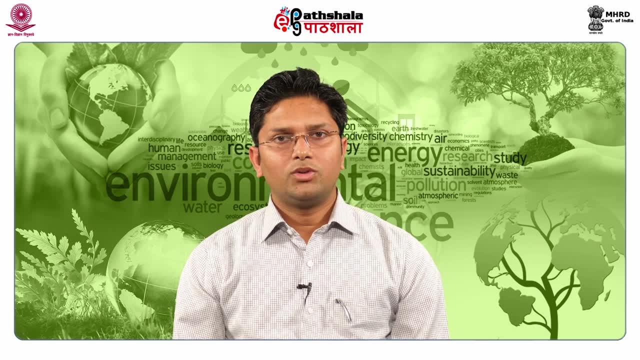 around 27.5 degree centigrade and which is thought to be an important threshold in producing rainfall. Now let us look how El Nino and La Nina events affects the Indian monsoon. Sir Gilbert Walker inferred that quantity of rainfall in the Indian subcontinent was often negligible in 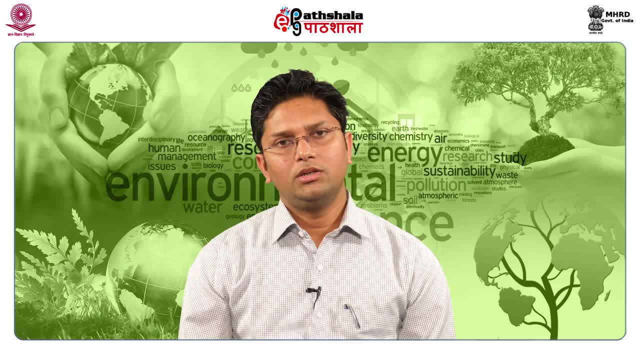 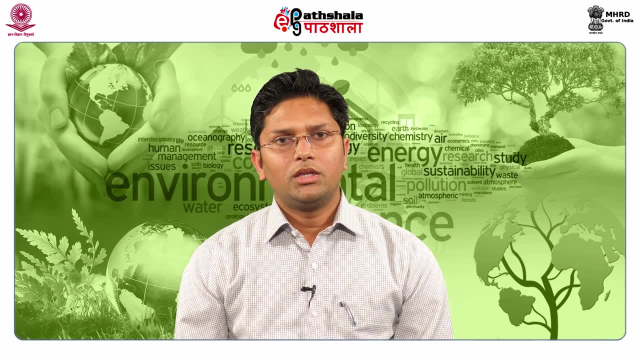 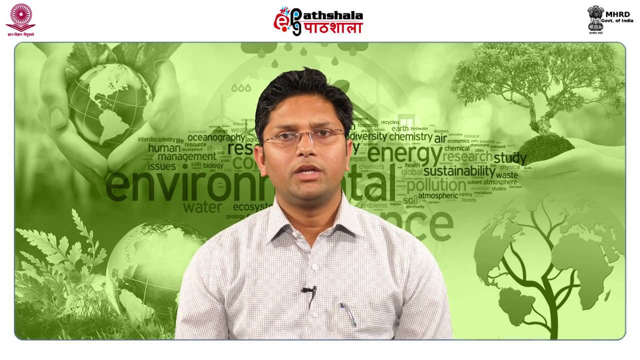 the years of high pressure at Darwin and corresponding low pressure at Tahiti. Conversely, low pressure at Darwin bore dwell for the precipitation quantity in India. Thus he established the relationship of southern oscillation with quantities of monsoon rains in India. The NSO is known to have a pronounced effect on the strength of southwest monsoon over India. with the monsoon being weak during the El Nino years. On the converse, La Nina years had particularly good monsoon strength over India. Kumar et al reported years with moderate to extreme cold state. That is when Nino 3 index is less than minus 1, have had abundant monsoon rains in India. 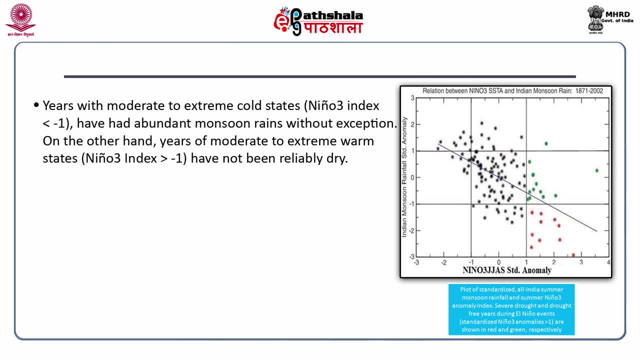 without exception. On the other hand, years of moderate to extreme warm states, that is, when Nino 3 index value is higher than minus 1, those years have not been really reliably dry. The six leading droughts since 1871 have occurred along with a standardized Nino 3. 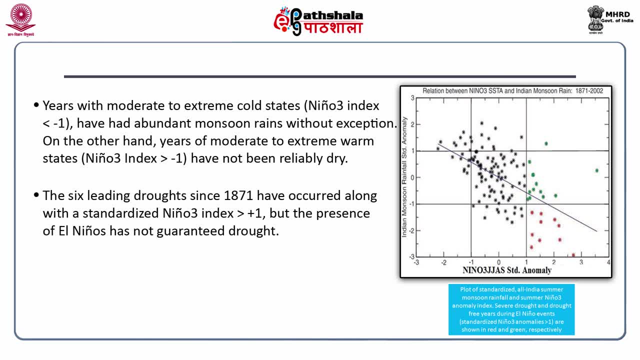 index value higher than plus 1.. The presence of El Nino has not guaranteed drought in India. In fact, there is no simple association that describes the relation between the Indian monsoon and Nino 3 sea surface temperatures when moderate to strong El Nino conditions exist. 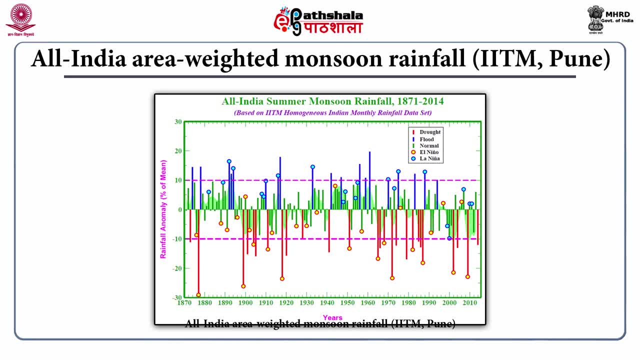 This figure is a plot of all India area-weighted mean summer monsoon rainfall published by IITM Pune. The long time series of this index, since 1871, have revealed several interesting aspects of the interannual and decadal scale variations in the monsoon, as well as its 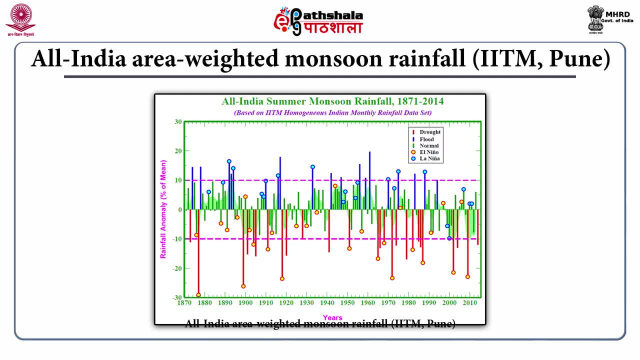 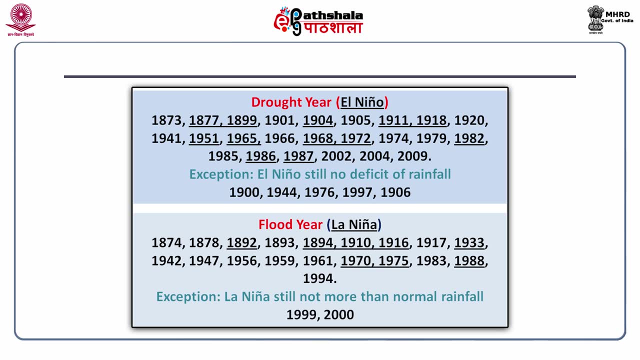 regional and global teleconnections. It is interesting to note that there have been alternating periods extending to three to four decades, with less and more frequent weak monsoons. over India, For example, the 44-year period between 1921 and 1964 witnessed just 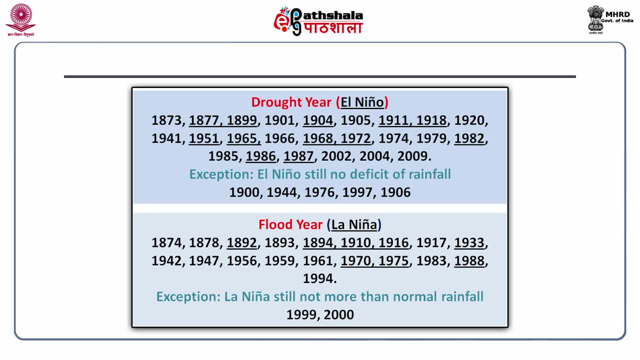 three drought years. During such a pause, the monsoon was found to be less correlated with NSO, Whereas during the other period, like 1950,, 1965 to 1987, it has only 10 drought years- The monsoon was found to be strongly linked with El Nino and southern oscillation. 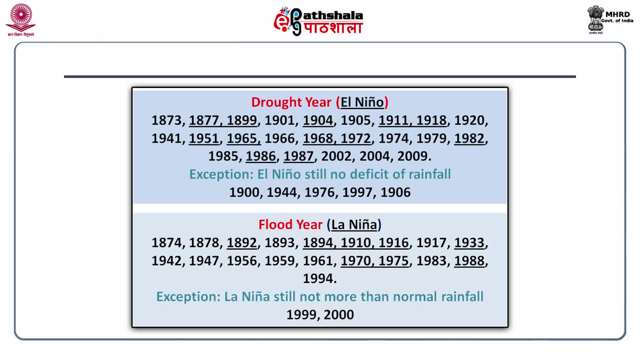 during this period, During the period 1871 to 2014,, there were 19 major floods in India. Here, flood has been defined as rainfall anomaly exceeding plus 10 percent. Usually, La Nina years in India caused more than normal summer monsoon rainfall, but there are years like 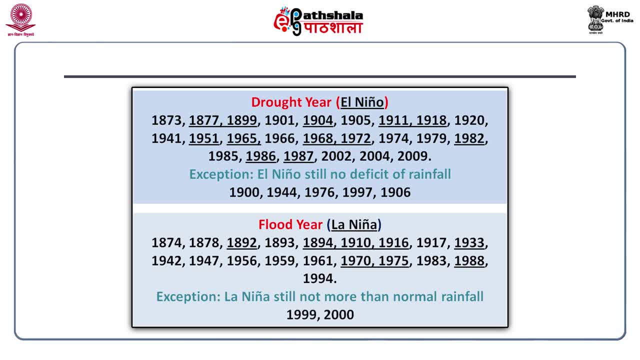 1990 and 2000, when the amount of rainfall was scanty or at least less than the normal rainfall. During the period 1871 to 2014,, there were 25 major drought years. Here the drought has been defined as when rainfall anomaly was minus 10 percent in terms of standard. 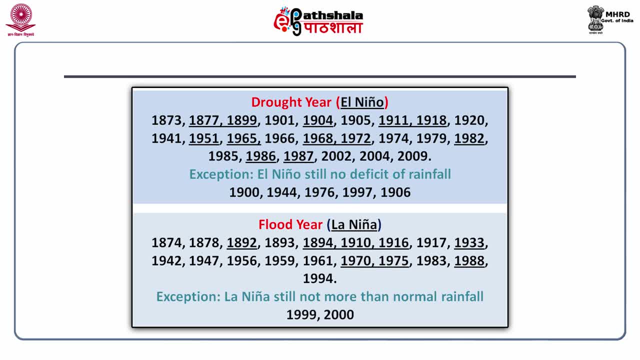 deviation. Usually El Nino years in India caused less than normal summer monsoon rainfall or drought like situations, but there are years like 1900, 1944, 1976, 1997 and 2006 when the amount of rainfall was abundant or at least more than the normal rainfall. This 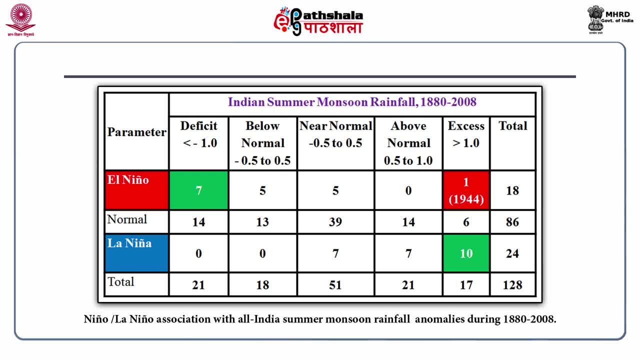 table gives another statistics for the period 1871 to 2014.. Out of this 128 years, 18 years were categorized as El Nino years, of which 7 had received deficient rainfall. Then 86 years was categorized as normal rainfall years. 24 years were categorized. 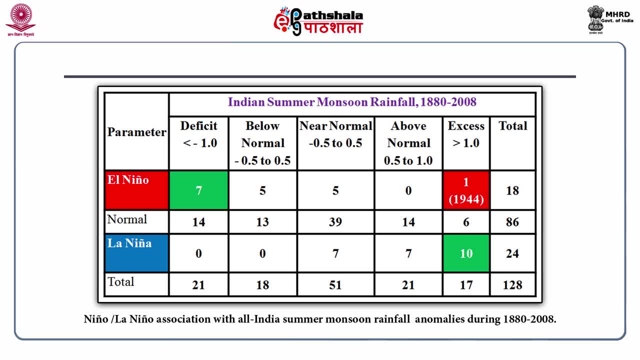 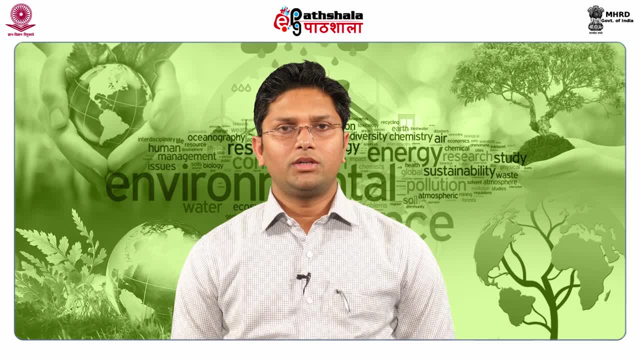 as La Nina years, but only in 10 years rainfall was excess, as per this index. To summarize, the coupling between ocean and atmosphere is straightforward. El Nino is an atmospheric anomaly. The large-scale anomaly of SST induces diabetic heating or cooling. 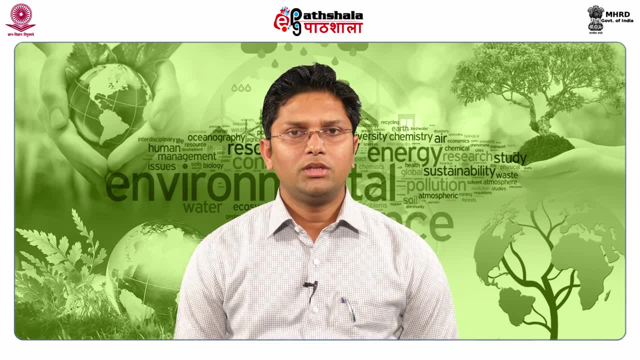 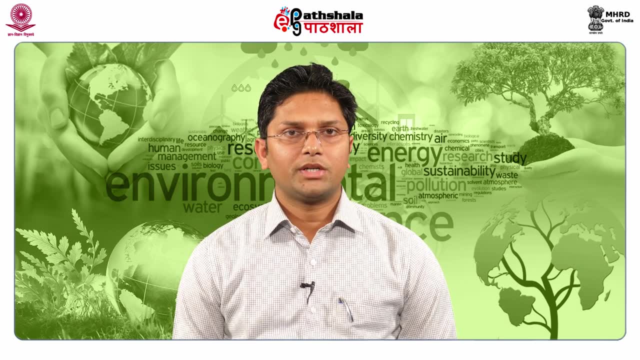 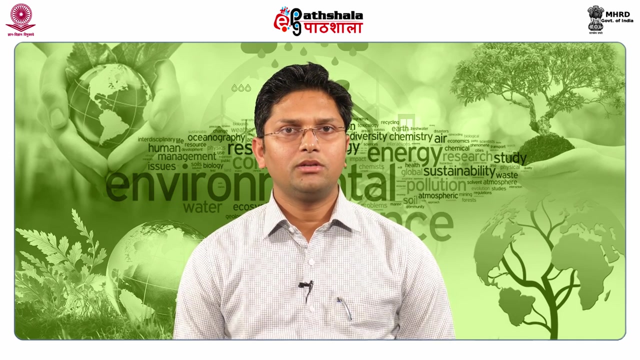 of the atmosphere, which modifies atmospheric circulation as well as the wind, stress and heat fluxes at the ocean surface. As a result, ocean thermal structure and circulation gets modified, giving rise to a series of positive feedbacks that strengthen the initial SST anomaly. El Nino and La Nina, both developed due to large-scale interaction of ocean and 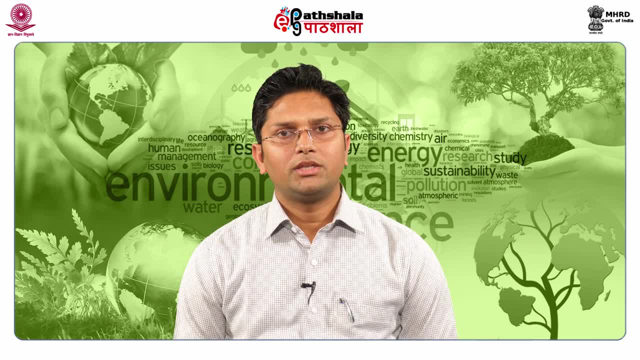 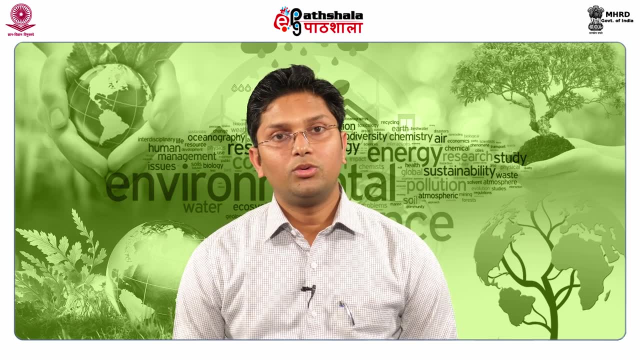 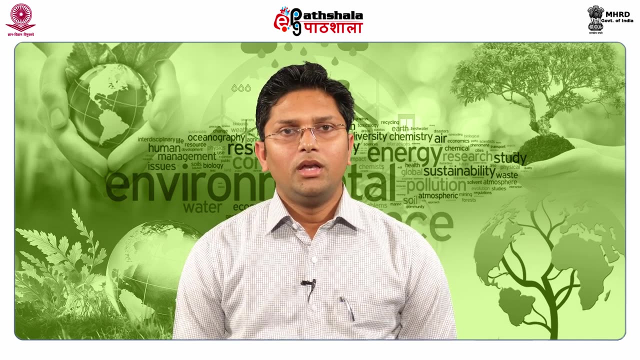 sphere. SST and sea surface pressure are the main drivers of these processes. Both of them have significant impact on a global scale due to teleconnection. The impacts of El Nino and La Nina are more devastating than the Fortuna El Nino episode is characterized.